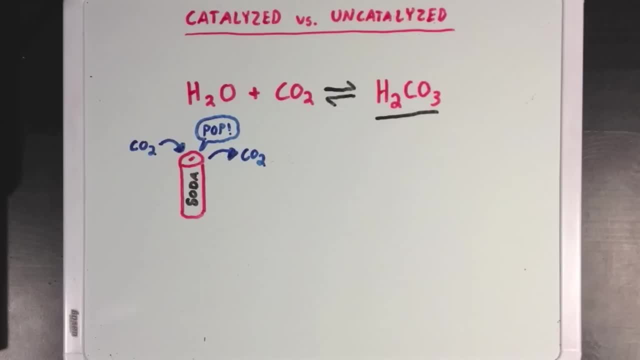 which is really just a bunch of CO2 escaping. But after that the soda will start to fizz really slowly And what's happening here is the carbonic acid that was made before is slowly dissociating back to carbon dioxide in water as CO2 escapes, And that extra CO2 that's being made will come out of the soda. 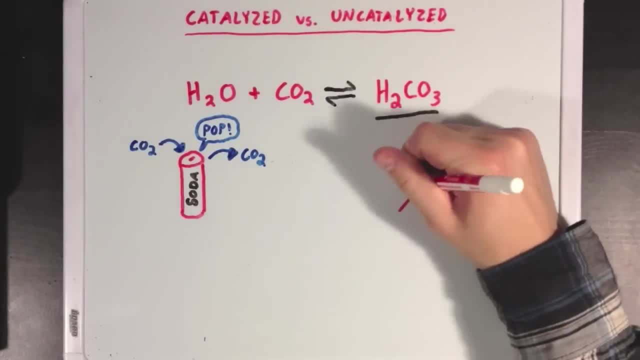 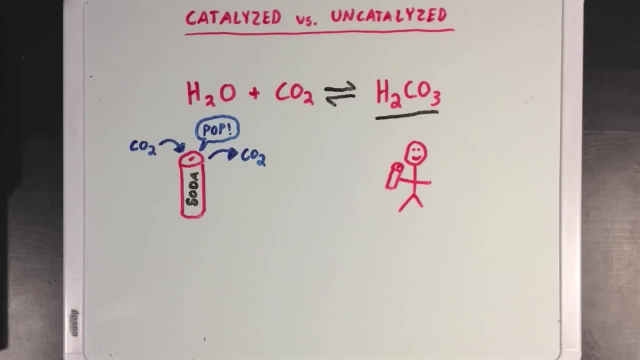 solution and you'll see it as little bubbles floating around. But what happens? if you then take this person over here and he'll pick up a can of soda and take a drink? That person might notice that the soda will start fizzing a lot more. 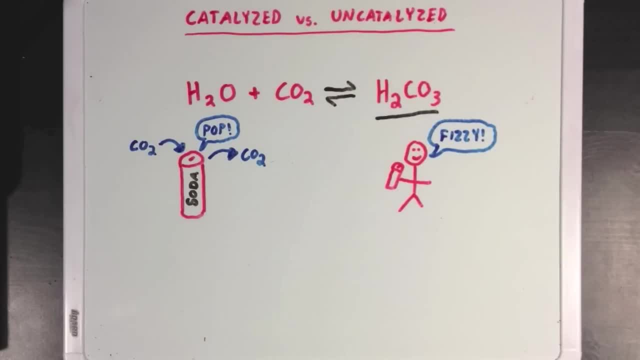 once it hits his or her tongue. And this is because humans have an enzyme in their blood and saliva called carbonic anhydrase, And this makes the carbonic acid turn into carbon dioxide in water much more quickly. So more CO2 will come out of the can and it'll fizz. 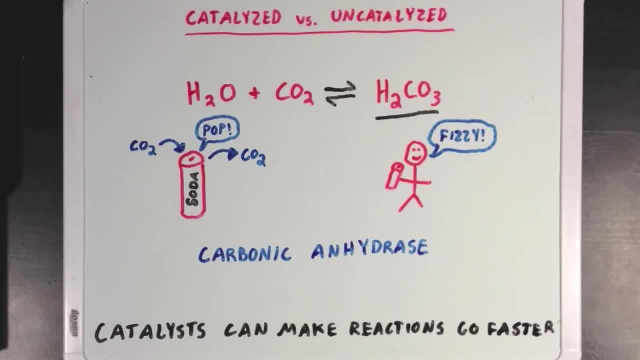 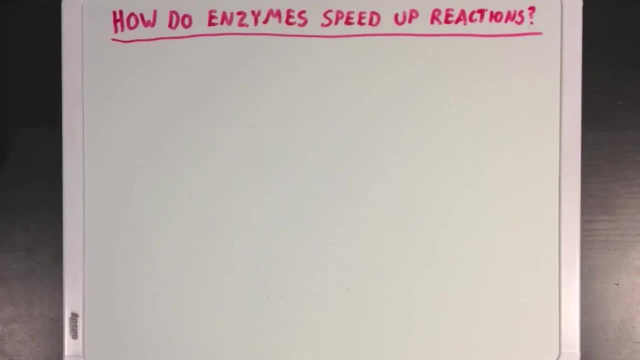 more, And this is just one of the many examples of how enzymes make reactions go faster. So how exactly do the enzymes make the reactions go faster though? Well, they use a bunch of different catalytic strategies to push reactions to a higher level of carbon dioxide, And they 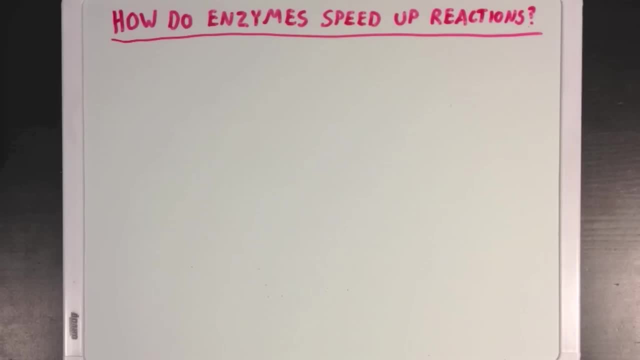 do so a little more quickly, And I'm going to talk about a few of those strategies just to give you an idea of what enzymes are doing. So first I'll mention acid-base catalysis, which happens when enzymes act like either acids or bases. Now remember that acids and bases are protons, donors and acceptors. 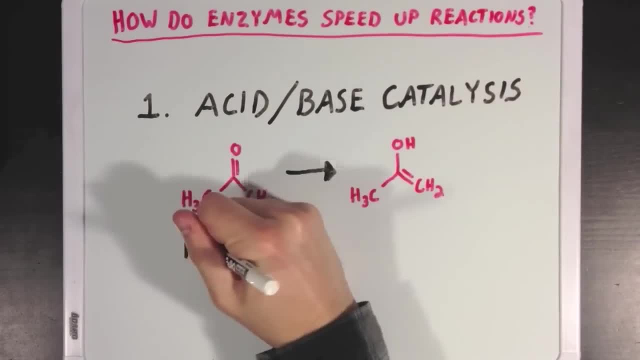 And if you look at this type of reaction which, if you remember from organic chemistry, is a ketoenol tautomerization reaction, we have a proton moving from a carbon atom to an oxygen atom And since acids and bases are pretty good proton carriers, they could both help with. 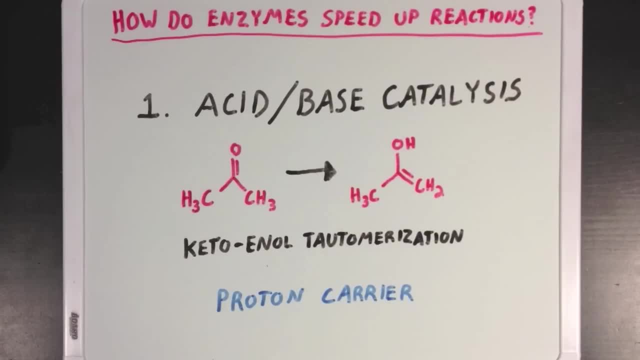 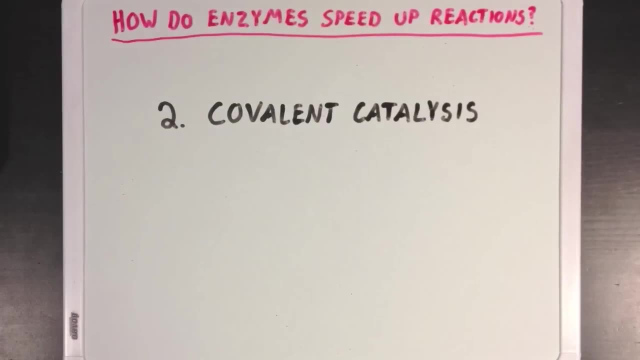 this reaction and make it go a little more quickly by helping to move that proton around instead of this molecule doing it by itself. Our next catalytic strategy is covalent catalysis, which happens when enzymes form a covalent bond with another molecule, usually their target molecule. Remember that covalent bonds. 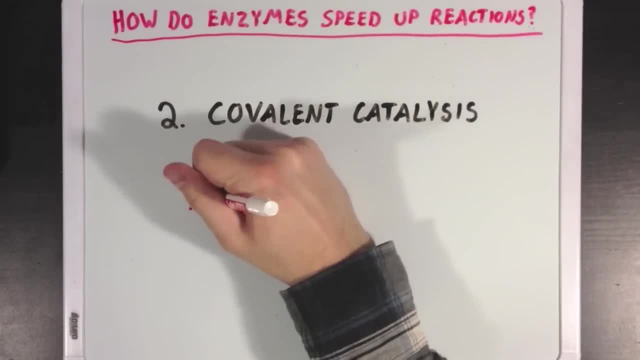 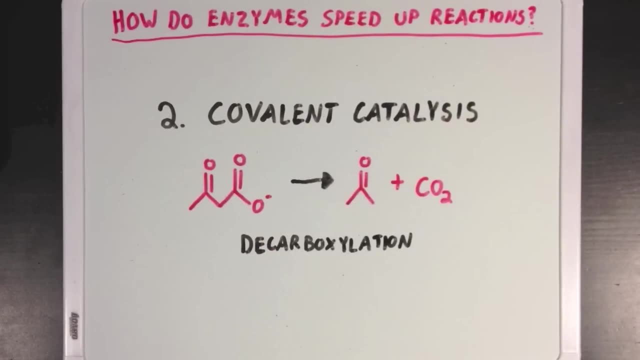 involve two molecules sharing electrons And looking at this reaction here we have a decarboxylation going on which, if you remember from organic chemistry, is when a carboxy or CO2 group is being taken off a molecule And, if you remember, these reactions usually have a lot of electrons moving around. So 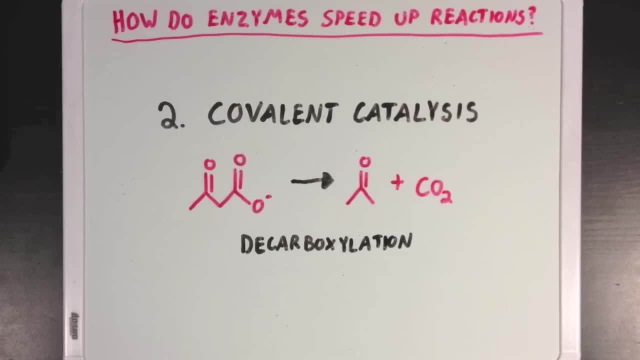 if we had a covalently bound enzyme that could hold onto some electrons and be an electron carrier, or what some people like to call an electron sink, then that would definitely help this type of reaction move a little more quickly. Next we have electrostatic catalysis. Now, if you remember, DNA is a very useful way to 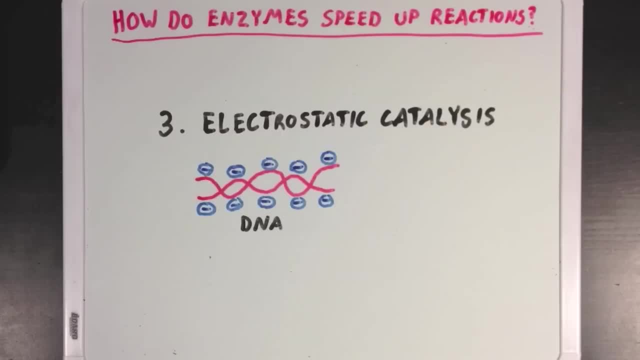 negatively charged polymer because of all the negatively charged phosphate groups that we find in DNA. So if an enzyme had a metal cation on it, like magnesium, we could use it to stabilize the negative charge found in DNA and make it a little easier to work with. 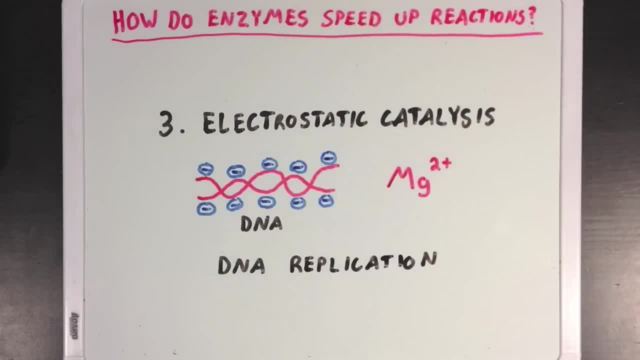 And DNA polymerase, which is the enzyme that allows DNA replication to occur, does exactly this, And in order for it to help with DNA replication, it needs to find a way to counteract all of the negative charge on DNA, and magnesium ions totally come in handy there. 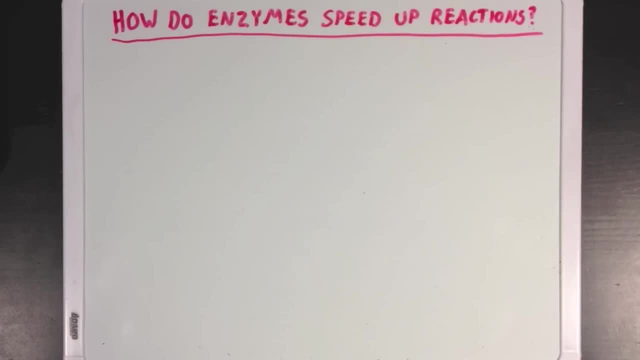 So the last catalytic strategy I want to mention is a little more general and it has to do with proximity and orientation effects. Remember that in order for two molecules to react with each other- which is usually what enzymes help out with- they need to physically collide at some point. 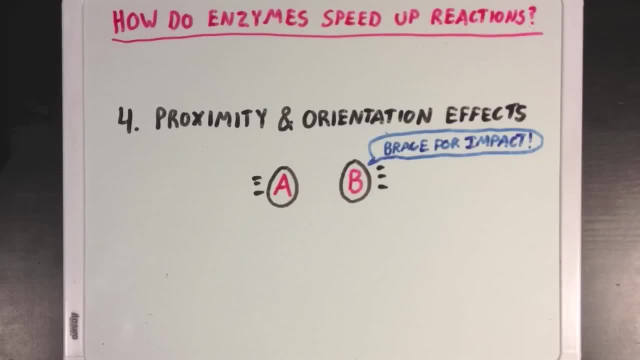 If we have molecule A and molecule B, they'll only react once they crash into each other, And a lot of enzymes are able to bring two molecules close together So that these types of collisions happen more often, making the two molecules react more quickly. 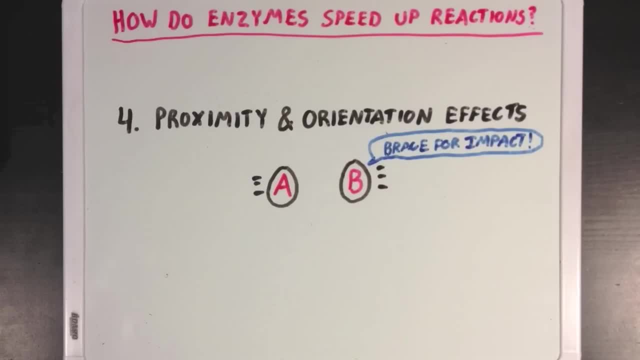 Also remember that the orientation of the two colliding molecules in space is also really important. If molecule A and molecule B collide, but one of them is upside down or not in the correct position, then the collision may not result in a successful reaction. 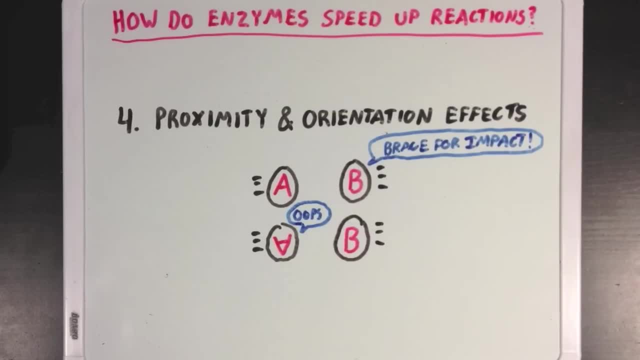 So enzymes also make sure that the two molecules will collide in the right orientation, And all of this makes sense. This increases the frequency of collision in general, but also helps to make sure that those collisions are successful and result in a reaction. So what did we learn? 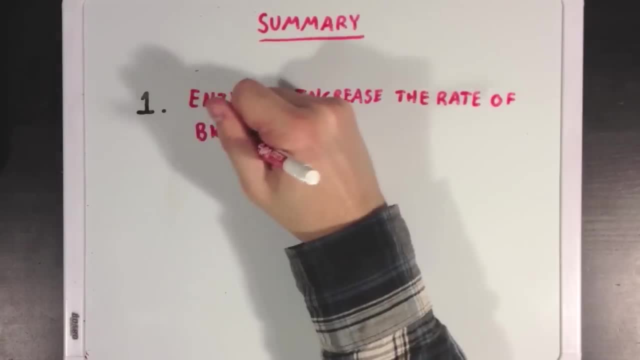 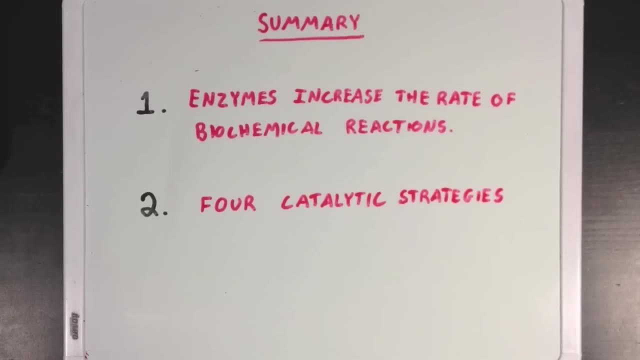 Well, first we learned that the role enzymes play is to make biochemical reactions happen more quickly, And the next thing we talked about were four of the many different catalytic strategies that enzymes can use. We talked about acid-base catalysis, which helps with proton transfer.